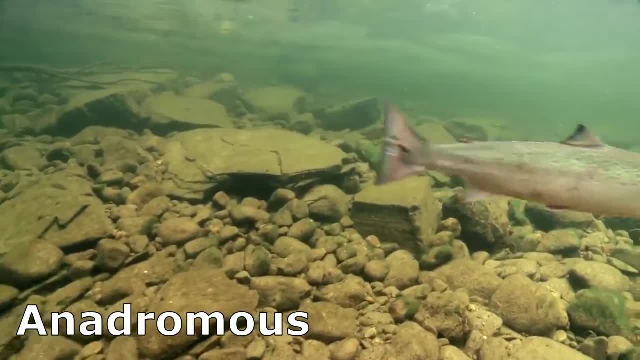 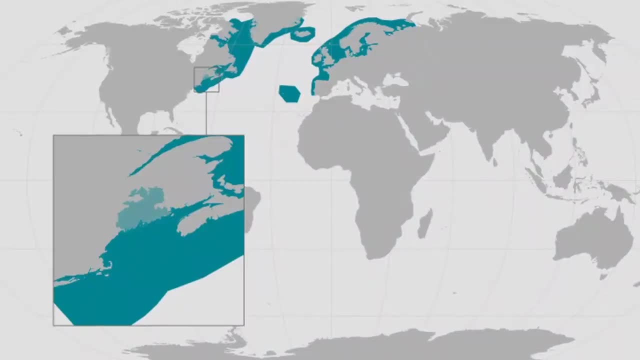 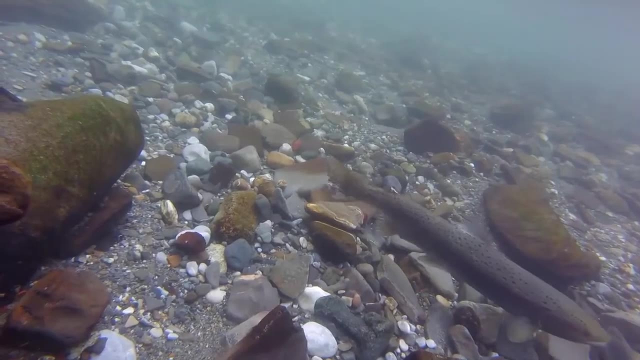 The Atlantic salmon is an anadromous species. This means that the adults live in the ocean and return to freshwater rivers to breed. These salmon can be found in the North Atlantic Ocean and the rivers that flow into it. Atlantic salmon spawn in freshwater in the fall. 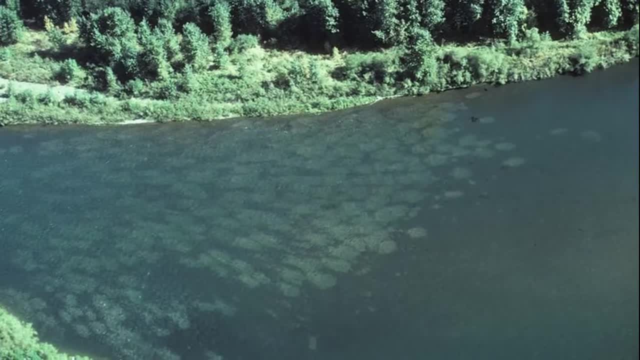 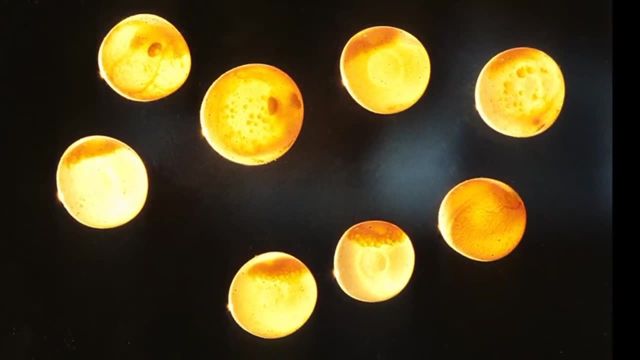 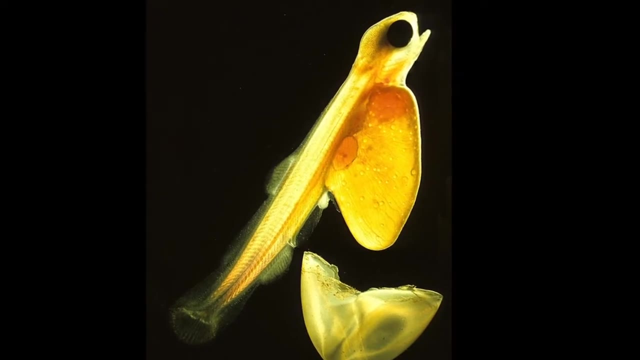 A female salmon will use its tail to dig a nest in the gravel where her eggs will be deposited. A female lays an average of 7,500 eggs. The gravel nest is called a red. Over the winter the eggs develop into small salmon called alevin. Alevin subsists on their. 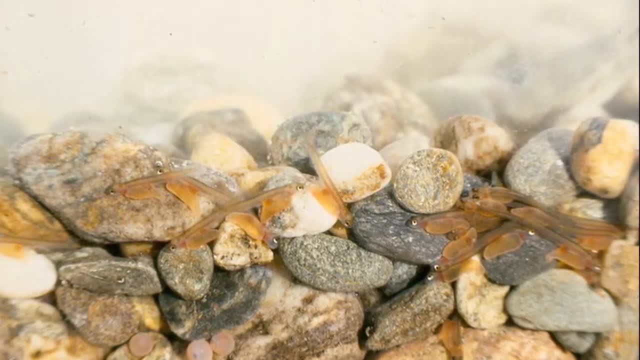 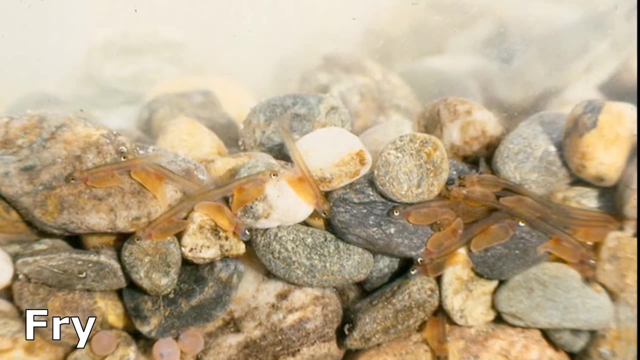 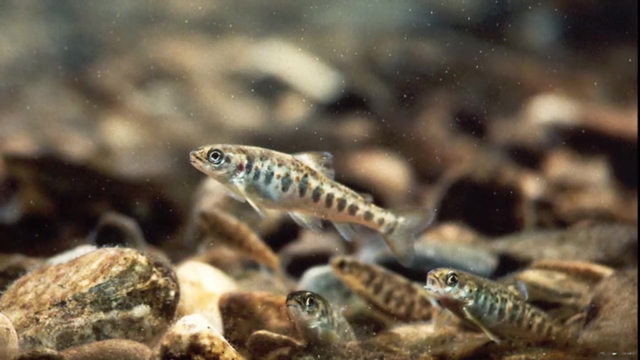 attached yolk sac. In May or June, after the yolk sac is depleted, the young salmon, now called fry, emerge from their nest. Only a small percentage of eggs survive. The fry develop into par with vertical stripes on their sides for camouflage Juvenile salmon. 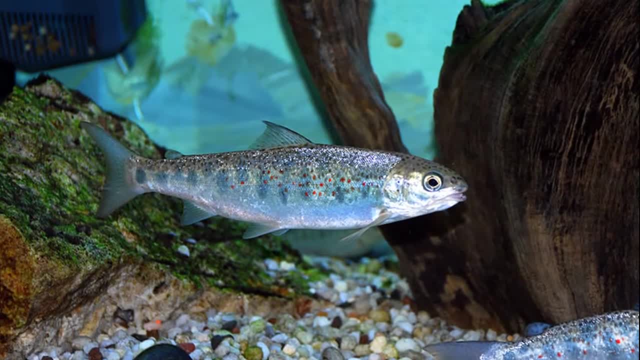 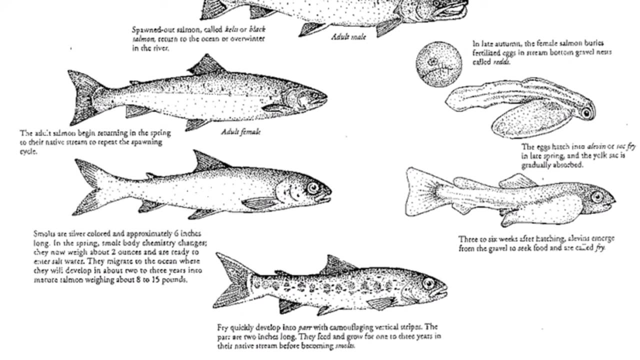 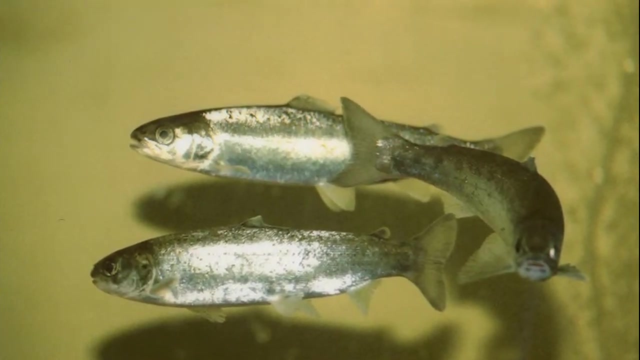 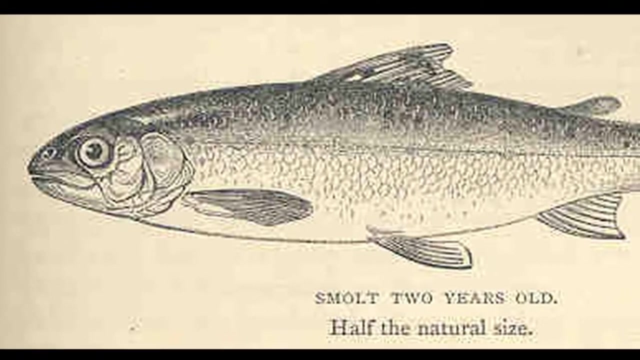 spend two or three years in freshwater before migrating to the ocean. Before migration, the salmon undergo a physiological transformation called smoltification. This transformation into smolts prepares the salmon for life in a marine habitat. During this process, their gills and organs change and the fish imprint on the chemical. 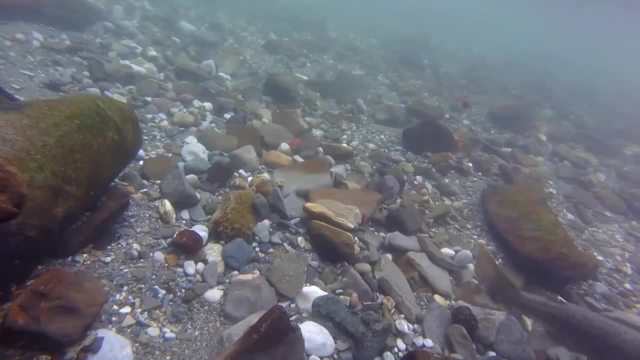 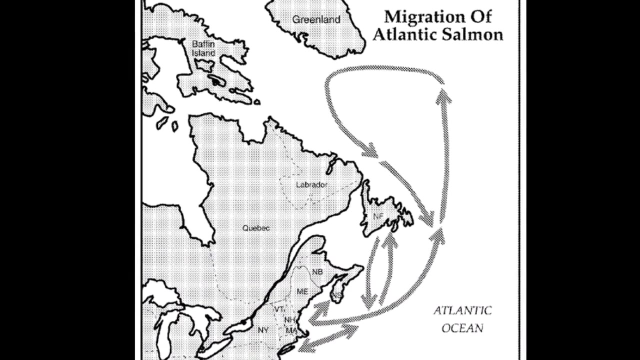 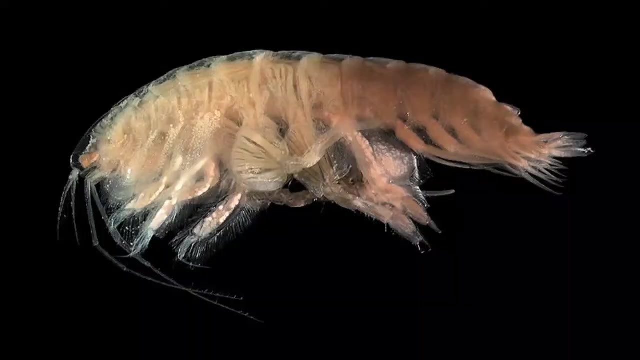 nature of the river. This enables them to find their way back to the place they were born. They migrate to the ocean to feed, grow and mature. The salmon grow much faster in saltwater than in freshwater. Adults prey on amphipods, krill and fish like kaplan. The salmon are 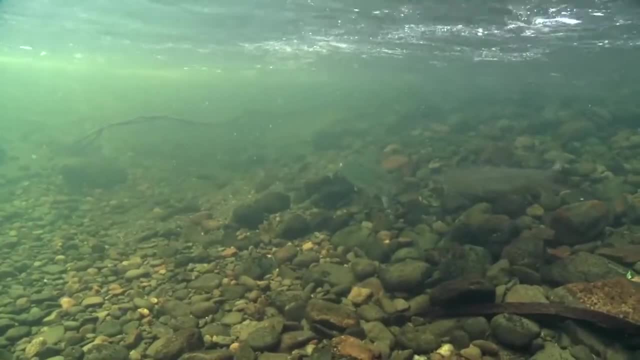 more prone to disease than to cancer. The salmon can also be found in the waters of the Atlantic. The salmon spend 1 to 3 years in the ocean, reaching 2 or 3 feet long, before returning to their natal rivers to spawn. 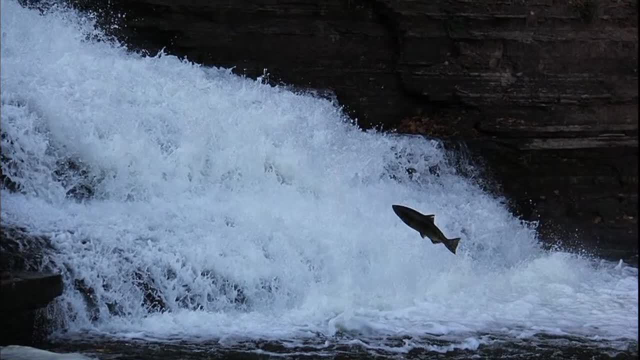 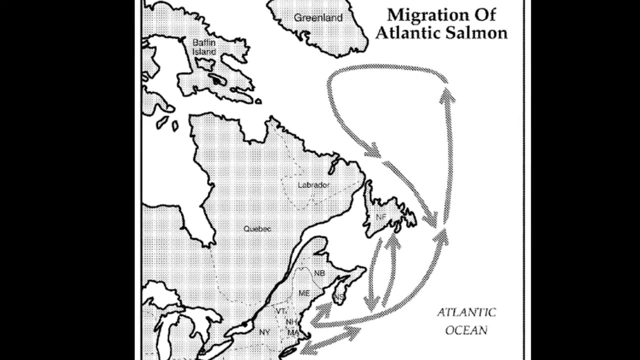 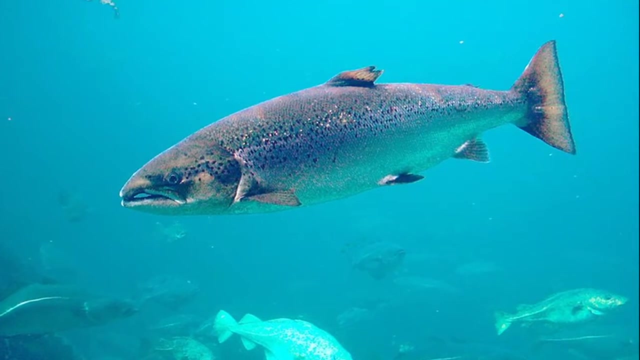 They must swim against strong river currents to reach their spawning grounds. They migrate with the help of the Earth's magnetic fields and their sense of smell. Many Atlantic salmon die after the first time they spawn. Very few spawn a second time, and even fewer a third or fourth time. 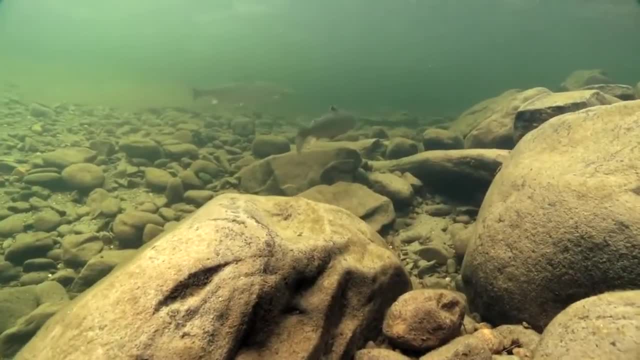 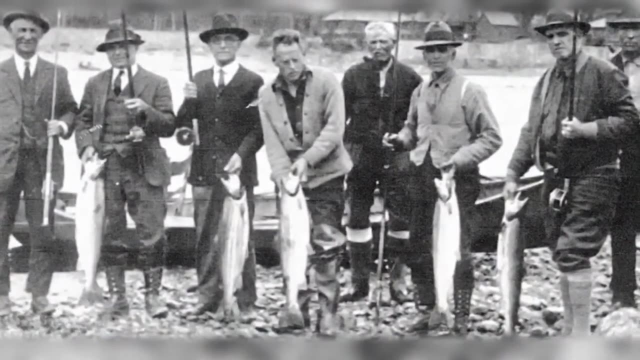 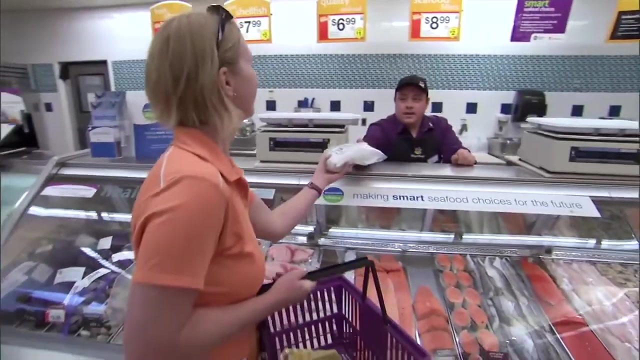 They only live 4 to 6 years. They are preyed on by birds, marine mammals and large fish. Commercial fishing for wild Atlantic salmon in the United States is prohibited. Only farm-raised Atlantic salmon can be found in the US fish markets. Atlantic salmon farming is controversial Because of the many environmental impacts. Chemicals and fish waste from these farms pollute water systems. The farms also rely on unsustainable industrial fishing to provide food for the salmon. Accidents sometimes happen, where thousands of farm fish are released into the ocean due to net failure. Even with fishing restrictions, many populations of wild Atlantic salmon are still in decline. Their populations are vulnerable to many threats, like pollution and predation by introduced species. Man-made dams and culverts can block access to their quality habitat. For more marine facts, click the SUBSCRIBE button. 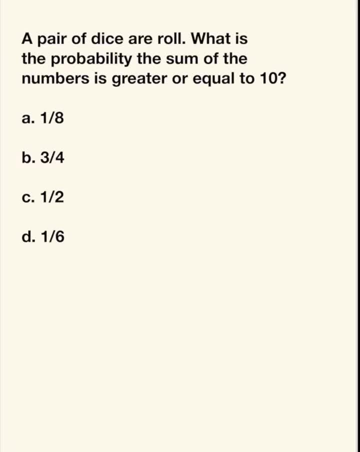 A pair of dice are rolled, What is the probability? the sum of the numbers is greater or equal to 10?? When you roll a pair of dice, you have six possibilities for the first dice and six possibilities for the second dice, giving you a total of 36 outcomes To get a sum that is greater. 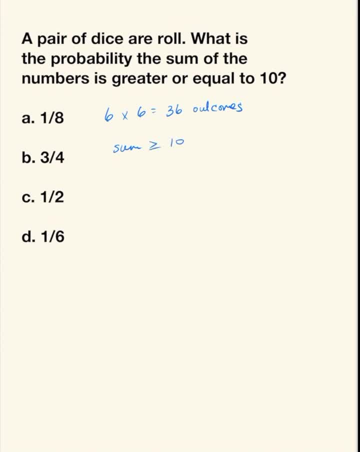 than or equal to 10,. you need to roll a 4 and a 6,, 6 and a 4,, 5 and a 5,, 5 and a 6,, 6 and a 5, and a 6 and a 6.. This is six different possibilities. The probability of getting a sum. 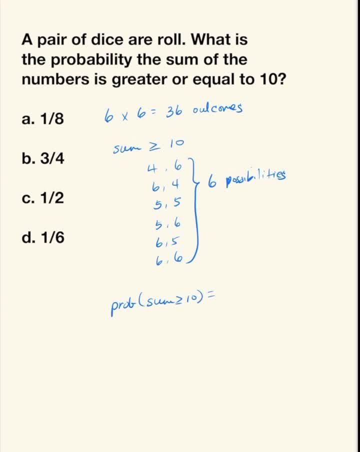 that's greater than or equal to 10 is equal to 6 over the total number of outcomes you can get, which is 36.. Now reduce that is equal to 1,6.. D- 약6.. D Was relieve 16-6.. So here we get an intrinsic value of 16 plus 16 and 105.. So you have something here that's greater than or equal to 10.. Let's round it up and figure out what the probability of getting a sum that is greater than or equal to 10 is greater than or equal to 10.. 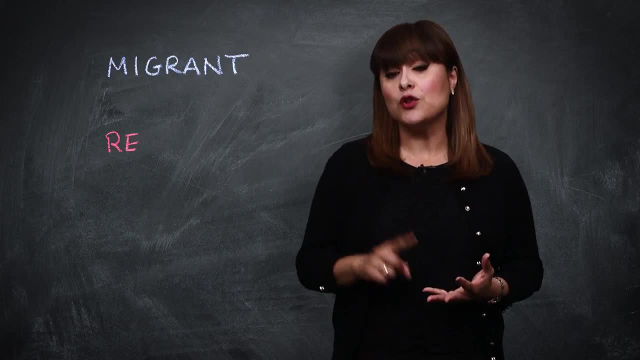 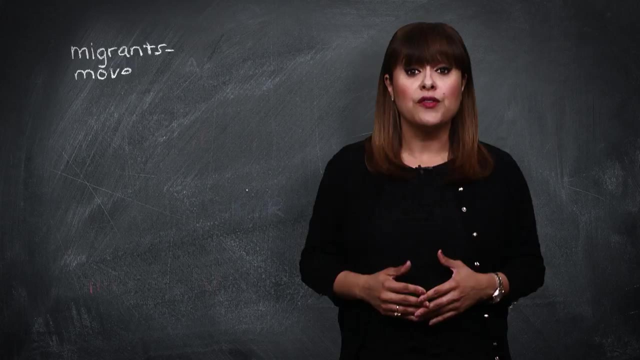 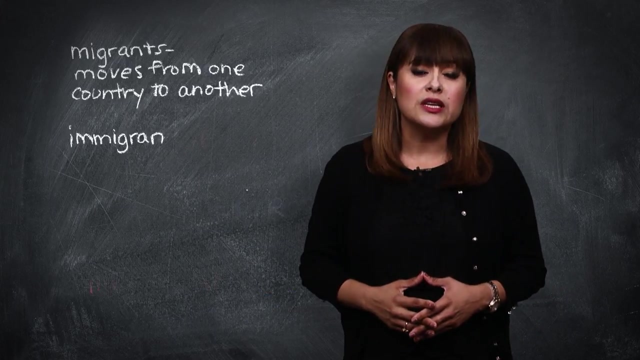 We hear these terms all the time: Migrant, refugee, asylum seeker, immigrant. What's the difference? Let's break it down. A migrant is a person moving from country to country for any number of reasons- Better life, better job, more opportunities. An immigrant is someone who moved. 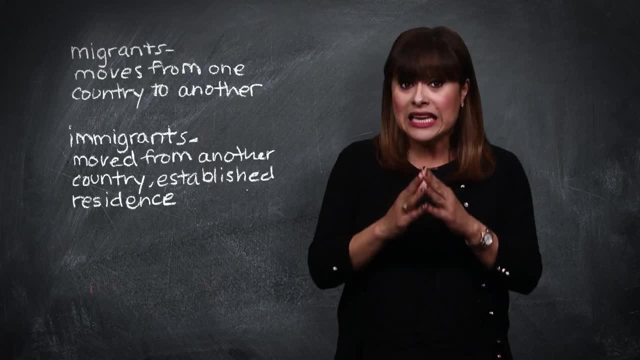 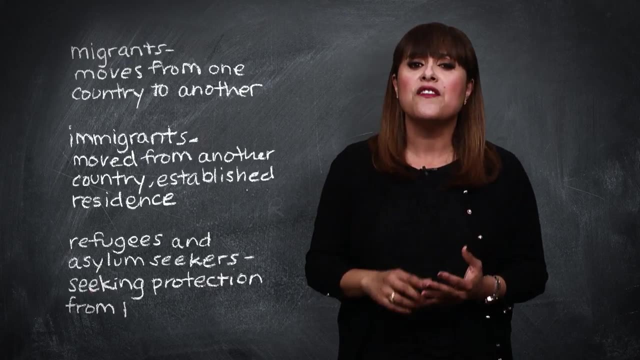 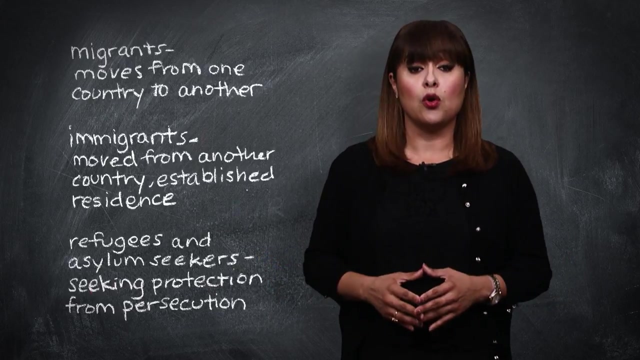 to another country and has established residency legally or illegally. Then there are refugees and asylum seekers. They both seek protection because they fear persecution based on a number of factors, including race, religion, membership in a particular social group or political opinion. But the process of how they get protection differs. Refugees must apply from overseas. 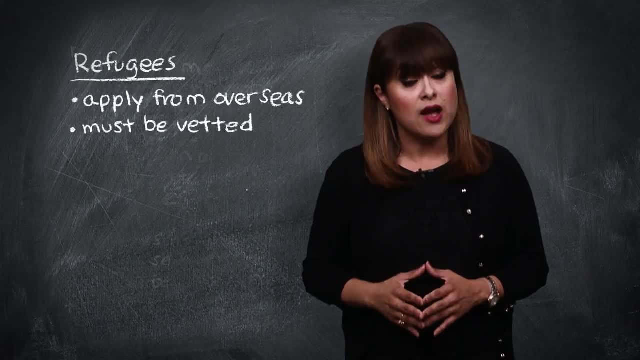 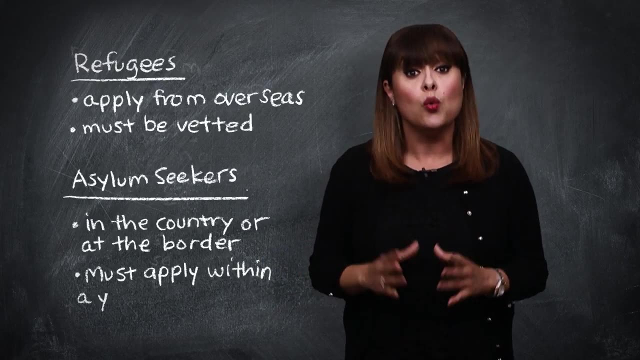 and have to be vetted and approved before traveling to the United States. Asylum seekers are people who are already in the US or at the border. They must apply for protection within one year of arriving. Whether you are a migrant or a refugee, you're a refugee and you're a